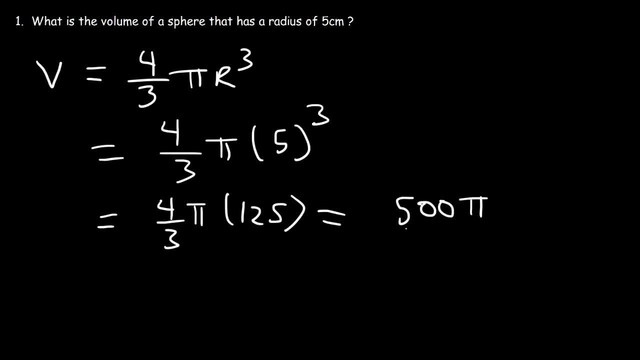 is 500. So the answer is 500 pi divided by 3 and the units cubic centimeters. If you want to get the decimal equivalent of that answer, just type it in your calculator: 500 pi over 3.. This is using the exact value of pi. by the way, It's 523.6 cubic. 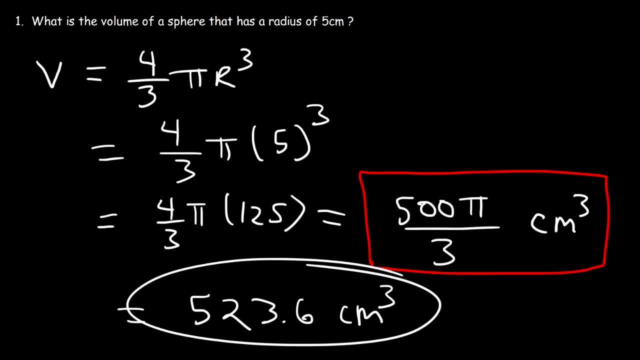 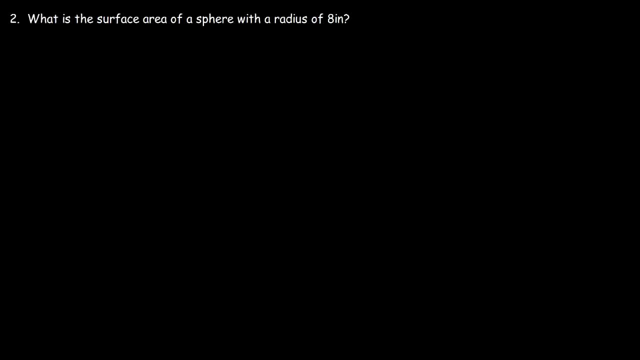 centimeters, So you can write your answer like that if you want to, But for the majority of this video I'm going to write the answer in terms of pi. Number two: What is the surface area of a sphere with a radius of 8 inches? 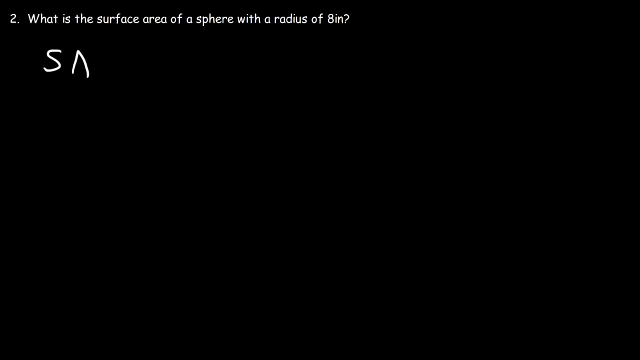 Well, let's begin by writing the formula first. The surface area is 4 pi times r squared, And we already have the value of r. It's 8 inches. So it's 4 pi times 8 squared, 8 squared or 8 times 8.. That's 64. And if you multiply 64 by 4, that's going to give. 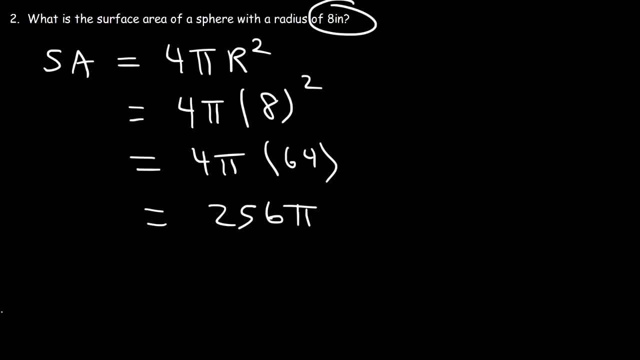 you 256.. So the answer is 256 pi. Now what are the units of surface area? In the case of volume, it could be inches, cubed, cubic feet, cubic yards, cubic something, Something raised to the third power. Now, whenever you're dealing with area, you're dealing with surface area. 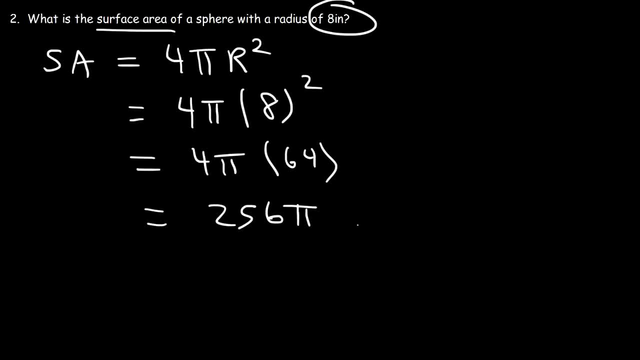 You're dealing with square units. In this case it's going to be inches, squared or square inches, So it's 256 pi square inches. Any type of area, It could be lateral area, surface area or just area in general, It's usually unit squared or square units. Number three: 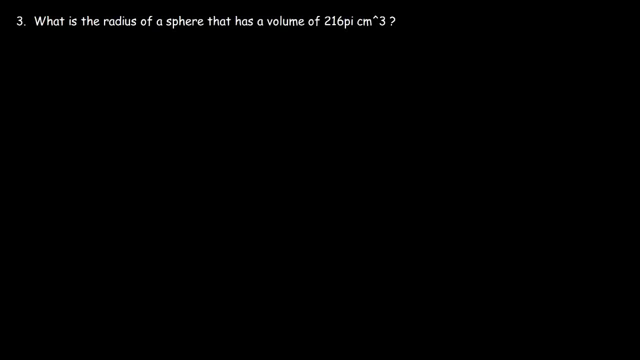 What is the radius of a sphere that has a volume of 216 pi cubic centimeters. So how can we find the radius, Given the volume of a sphere? Well, we need to write an equation that connects the volume and the radius of the sphere. So it has to be this one. 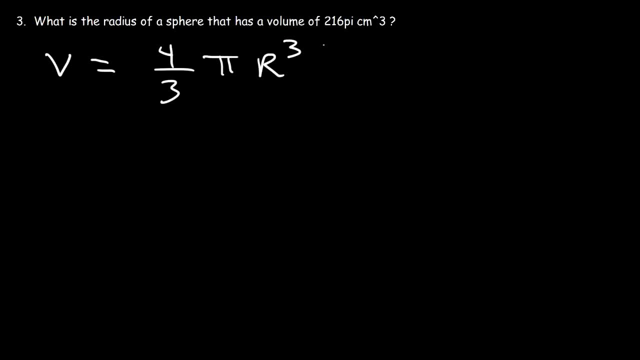 V is equal to 4 thirds times pi times r cubed. So we have the value of V. It's 216 pi, And our goal is to find the value of r. The first thing we could do is divide both sides by pi, So we could cancel that if we want to. 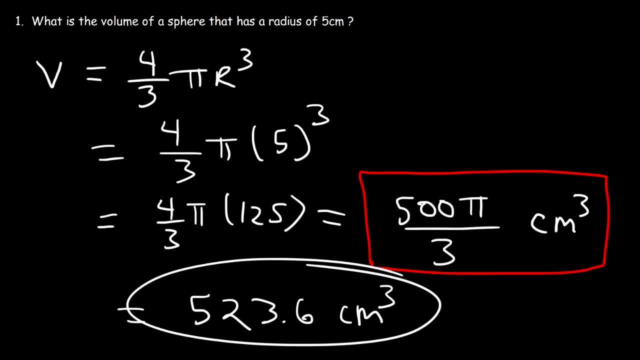 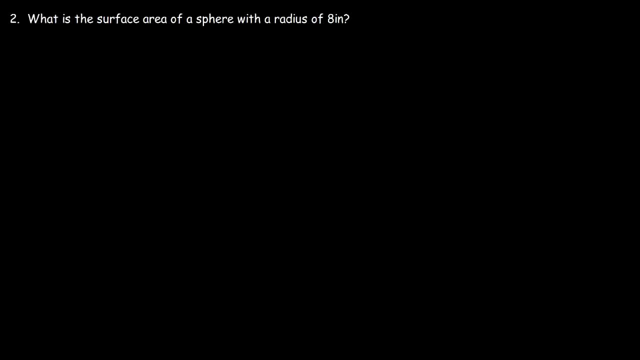 centimeters, So you can write your answer like that if you want to, But for the majority of this video I'm going to write the answer in terms of pi. Number two: What is the surface area of a sphere with a radius of 8 inches? 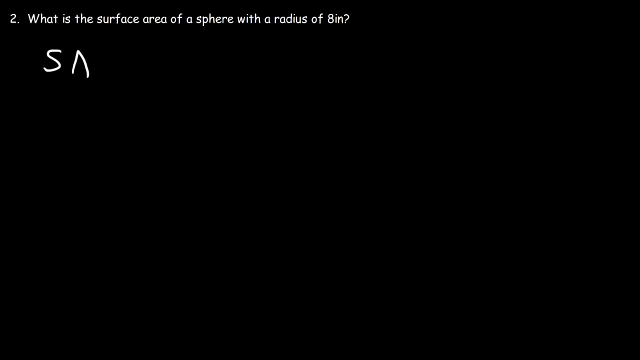 Well, let's begin by writing the formula first. The surface area is 4 pi times r squared, And we already have the value of r. It's 8 inches. So it's 4 pi times 8 squared. 8 squared, or 8 times 8, that's 64. And if you multiply 64 by 4, that's going to give. 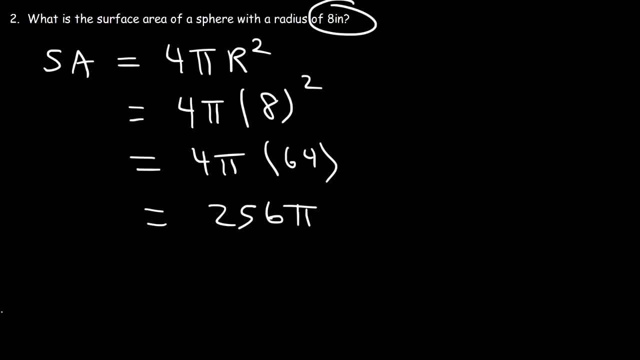 you 256.. So the answer is 256 pi. Now what are the units of surface area? In the case of volume, it could be inches, cubed, cubic feet, cubic yards, cubic something, Something raised to the third power. Now, whenever you're dealing with area, you're dealing with surface area. 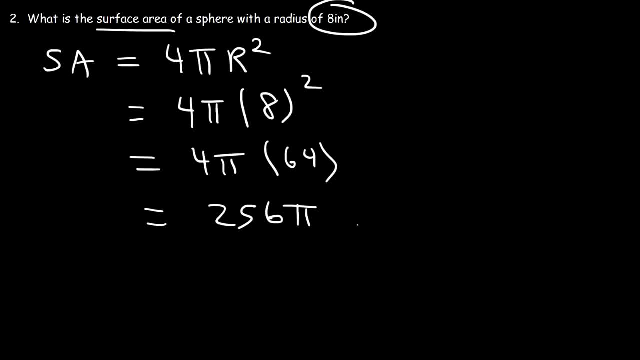 You're dealing with square units. In this case it's going to be inches, squared or square inches, So it's 256 pi square inches. Any type of area, It could be lateral area, surface area or just area. in general, It's usually unit squared or square units. 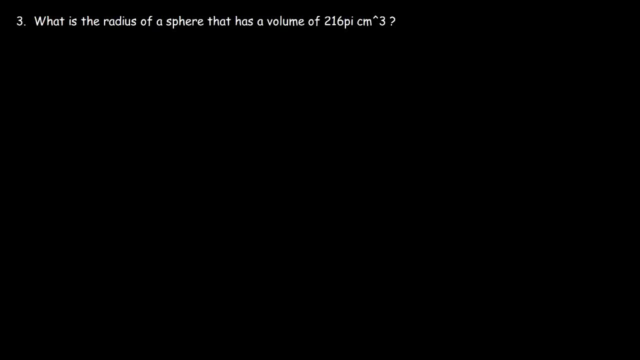 Number three: What is the radius of a sphere that has a volume of 216 pi cubic centimeters? So how can we find the radius, given the volume of a sphere? Well, we need to write an equation that connects the volume and the radius of the sphere. So it has to be this one: V is equal to four-thirds times pi times r. 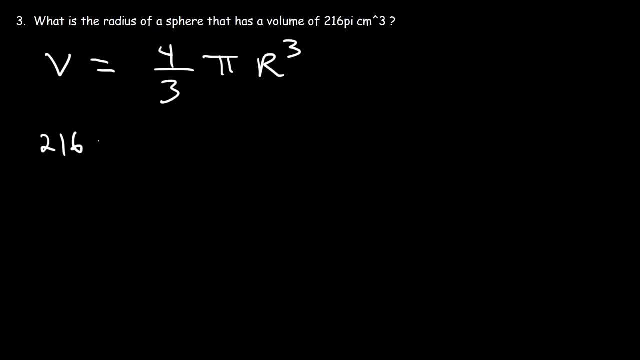 cubed. So we have the value of V. It's 216 pi, And our goal is to find the value of r. The first thing we could do is divide both sides by pi, So we could cancel that if we want to. Next, let's: 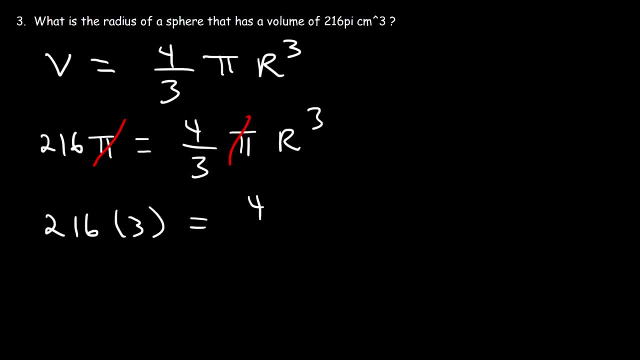 multiply both sides by three just to get rid of the fraction on the right side. If we multiply both sides by three, these will cancel Now 216 times three. we know that 200 times three is 600, and 16 times three is 48.. So this is going to be 648.. That's equal to four r cubed. 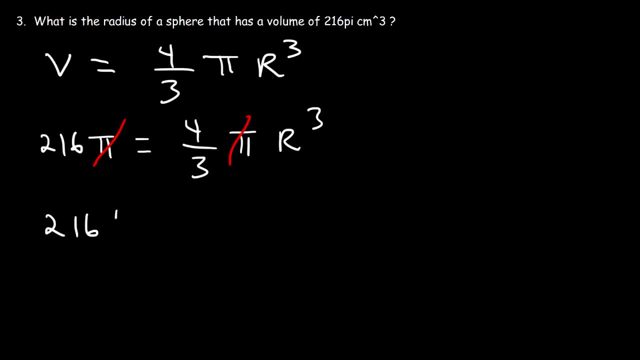 Next, let's multiply both sides by 3.. Just to get rid of the fraction on the right side: If we multiply both sides by 3, these will cancel Now 216 times 3.. We know that 200 times 3 is 600.. And 16 times 3 is 48. So this is going to be 648. That's equal to 4 r cubed. Now let's divide both sides by 4.. 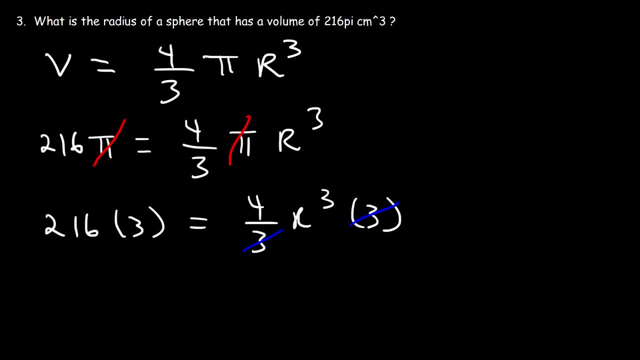 Now let's divide both sides by 4.. 600 divided by 4 is 150. And 48 divided by 4 is 12.. So if you add 150 and 12, you should get 162.. So 162 is equal to r cubed. 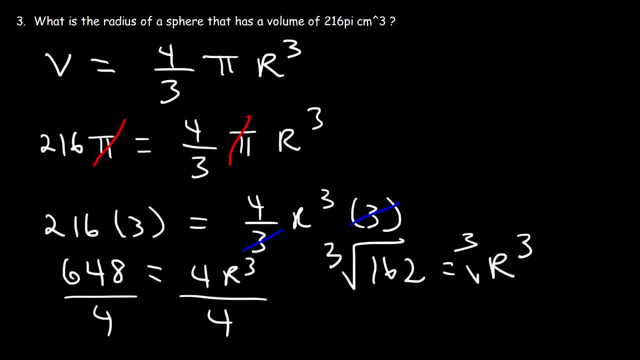 So now we need to take the cube root of both sides, So these will cancel, And so r is equal to the cube root of 162.. Now you can type this in your notebook. You can type this in your calculator as 162 raised to the 1 third, if you want to. 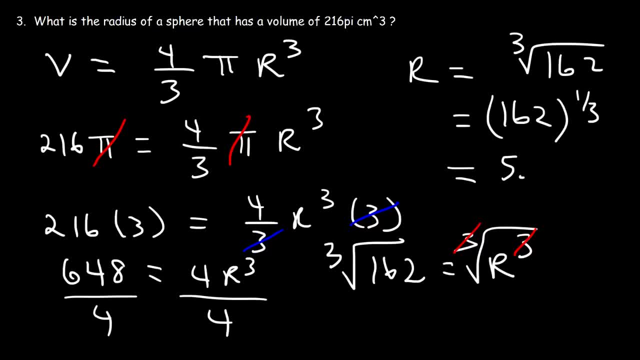 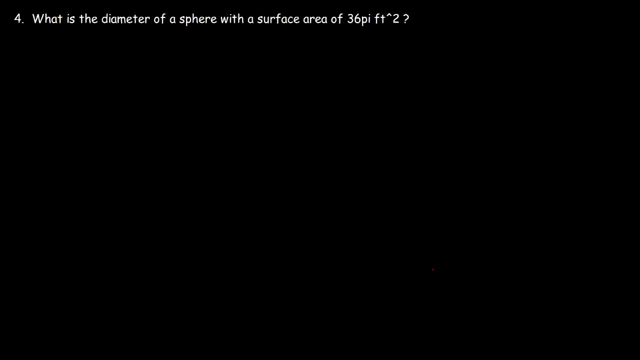 And you should get about 5.45.. And the units will be centimeters. So that's the length of the radius of the sphere. That's how you could find it, Number 4.. What is the diameter of a sphere with a surface area of 36 pi square feet? 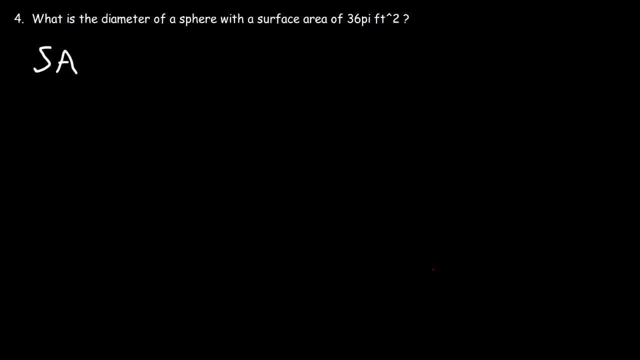 Using this formula, We could find the radius. The surface area is 4 pi r squared. And once we have the radius, we could find the diameter. The diameter is simply 2r. So let's say, if you have a circle with radius r, 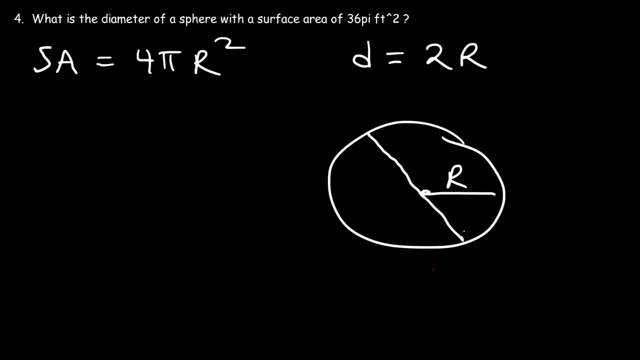 The diameter is basically twice the radius. It's from one end to the other end and it passes through the center of the circle or sphere. Now let's go ahead and find the radius first. So the surface area is 36 pi. So let's cancel pi. 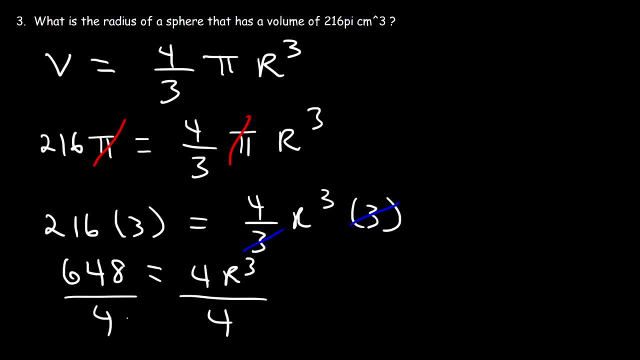 Now let's divide both sides by four. 600 divided by four is 150, and 48 divided by four is 12.. So if you add 150 and 12, you should get 162.. So 162 is equal to r cubed. 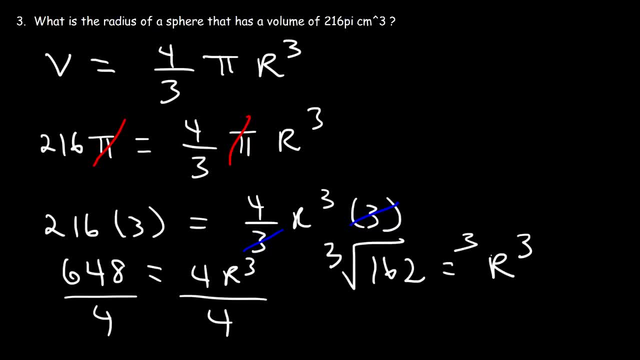 So now we need to take the cube root of both sides, So these will cancel, And so r is equal to the cube root of 162.. Now you can type this in your calculator as 162 raised to the one-third, if you want to, And you should get about 5.45, and the units will be. 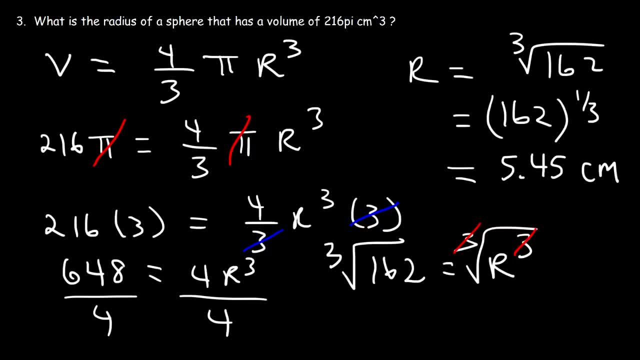 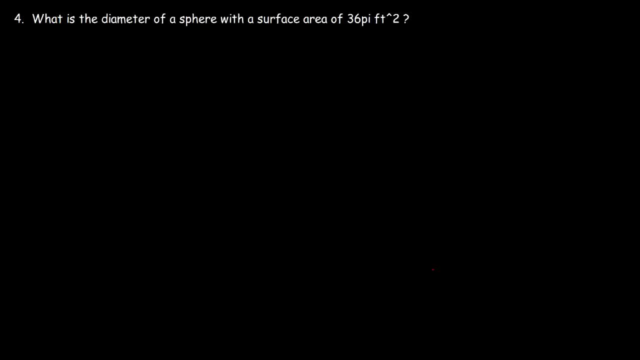 centimeters. So that's the length of the radius of the sphere. That's how you could find it. Number four: What is the diameter of a sphere with a surface area of 36 pi squared? Using this formula we could find the radius. The surface area is 4 pi r squared. 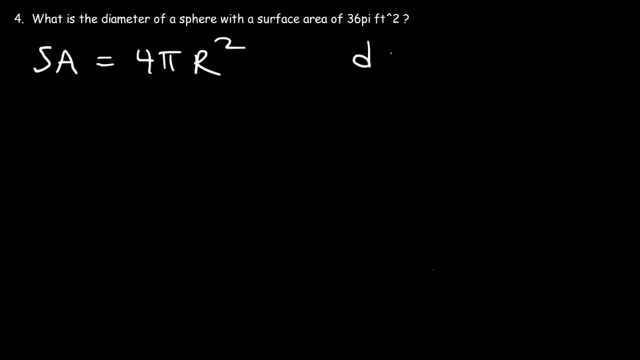 And once we have the radius, we could find the diameter. The diameter is simply 2r. So let's say, if you have a circle with radius r, the diameter is basically twice the radius. It's from one end to the other end and it passes through the center of the circle. 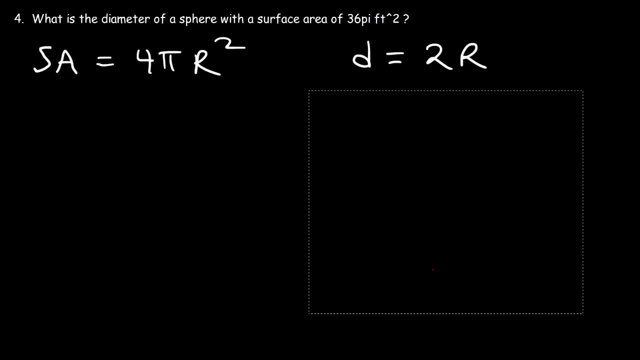 Or a sphere. Now let's go ahead and find the radius first. So the surface area is 36 pi. So let's cancel pi And then let's divide both sides by 4.. 36 divided by 4 is 9.. 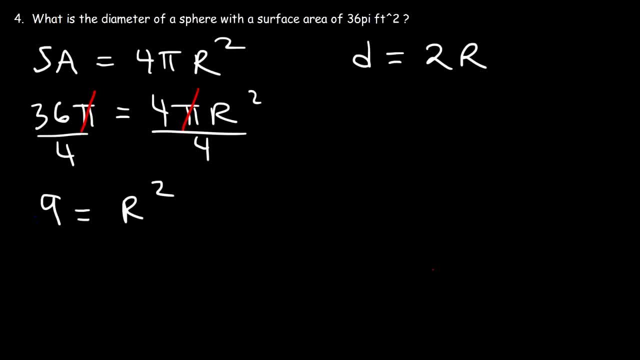 So 9 is equal to r squared. Now let's take the square root of both sides. So 9 is equal to 4 r squared sides. so the radius is 3 feet long and the diameter is twice the length of the radius. so it's gonna be 2 times 3. therefore the diameter is 6 feet long. 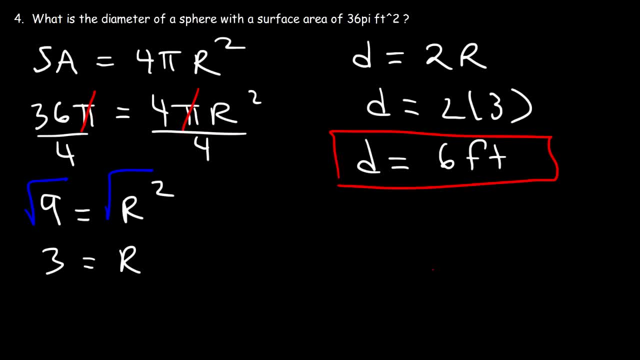 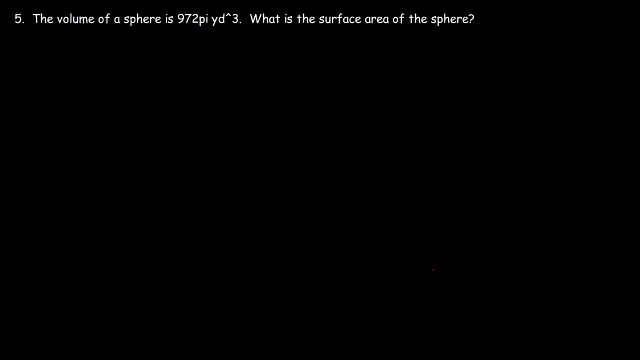 and so that's how you could find the diameter of a sphere. here's another one that we can work on, number 5: the volume of a sphere is 972 pi cubic yards. what is the surface area of the sphere? so how can we find the surface area if we're 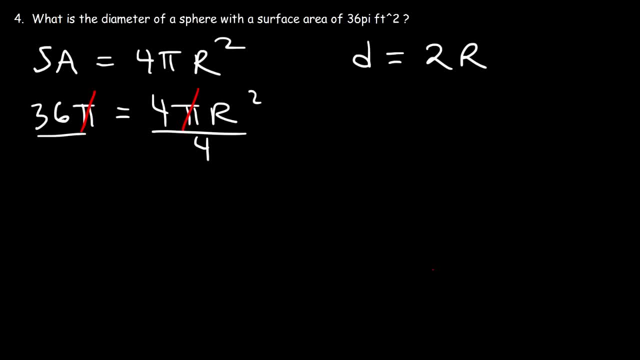 And then let's divide both sides by 4.. 36 divided by 4 is 9.. So 9 is equal to r squared. Now let's take the square root of both sides, So the radius is 3 feet long And the diameter is twice the length of the radius. 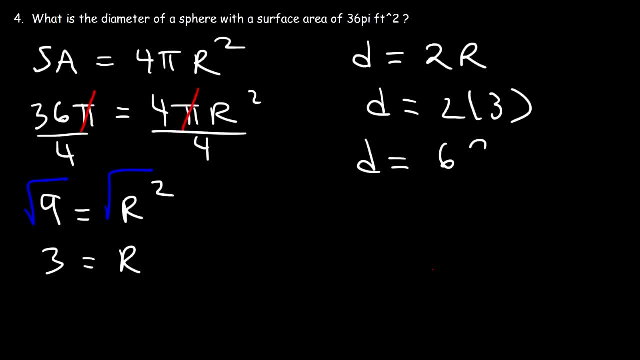 So it's going to be 2 times 3.. Therefore, the diameter is 6 feet long, And so that's how you could find the diameter of a sphere. Here's another one that we could work on, Number 5.. The volume of a sphere is 972 pi cubic yards. 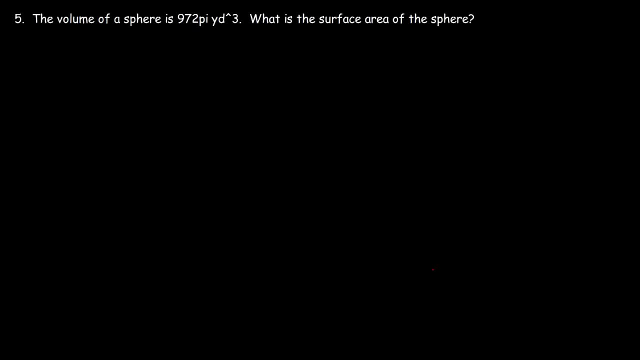 What is the surface area of the sphere? So how can we find the surface area if we're given the volume of a sphere? Well, we need to use both equations that we know: V is equal to 4 thirds pi r cubed And the surface area is 4 pi r squared. 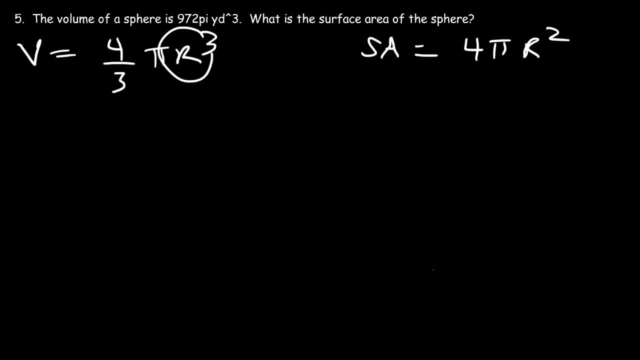 We have the volume already. We need to use the first equation to find r. Once we can find r, we can plug it into the second equation to get the surface area. So let's work with the first equation. So V is 972 pi. 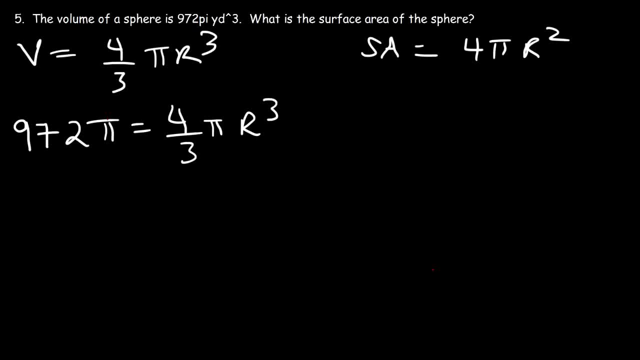 So the first thing that we need to do is cancel pi, since it's on both sides. Now, what do you think we need to do next? What's our next step? What I prefer to do is to multiply both sides by 3. So these can be cancelled. 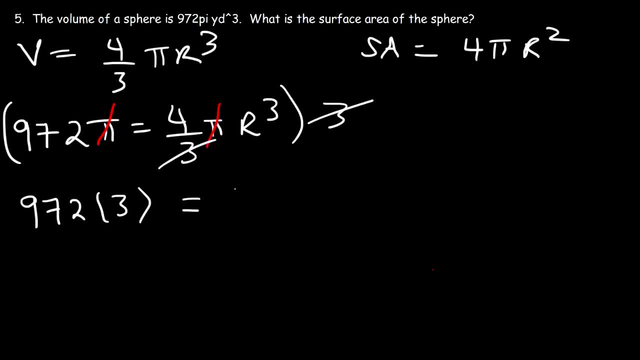 On the left side it's going to be 972 times 3. And that's equal to 4 times r. cubed 972 times 3, that's 2916.. Next we need to divide both sides by 4.. 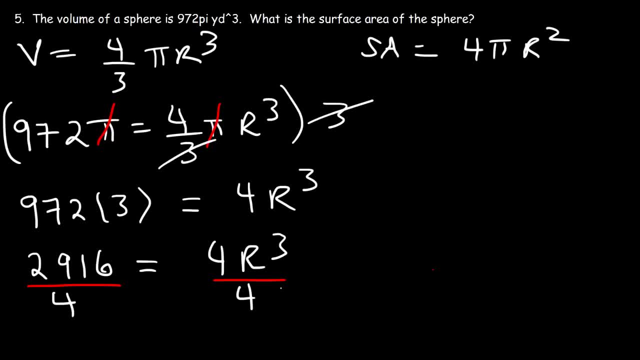 So we can get r cubed by itself: 2916 divided by 4 is 729.. So that's equal to r cubed. Now, at this point we need to take the cube root of both sides, 729 raised to the 1 over 3, which is the cube root of 729. 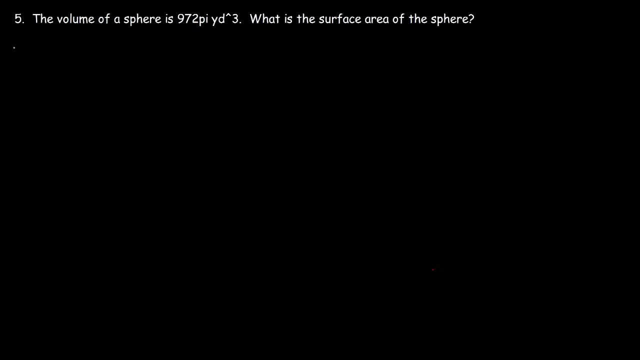 given the volume of a sphere. well, we need to use both equations that we know. V is equal to 4 thirds pi R cubed and the surface area is 4 pi R squared. we have the volume ready. we need to use the first equation to find R, once we could. 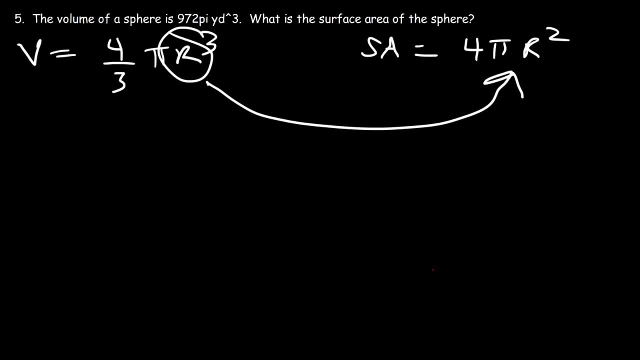 find R, we could plug it into the second equation to get the surface area. so let's work with the first equation. so V is 972 pi. so the first thing that we need to do is cancel pi, since it's on both sides. now what do you think we need to do next? what's our next step? what I 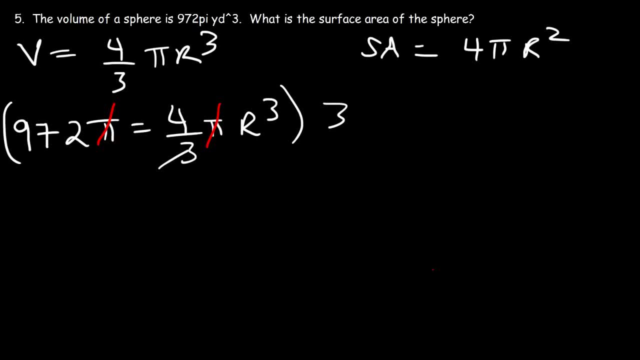 prefer to do is to multiply both sides by 3 so these can be cancelled. on the left side is going to be 972 times 3, and that's equal to 4 times R. cubed 972 times 3, that's 2,916. next we need to divide both sides by 4 so we can get. 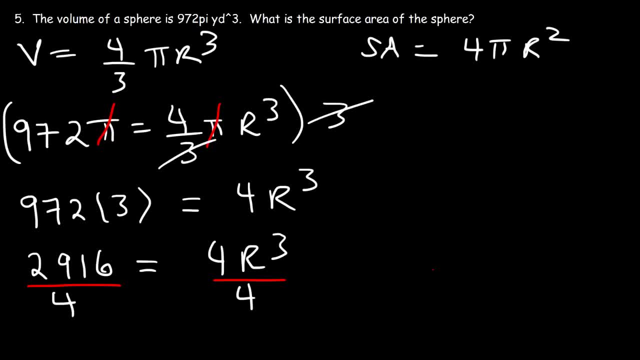 R cubed by itself, 2916 divided by 4 is 729, so that's equal to R cubed. now, at this point we need to take the cube root of both sides: 729 raised to the 1 over 3, which is the cube root of 729, that's equal to 9, so 9. 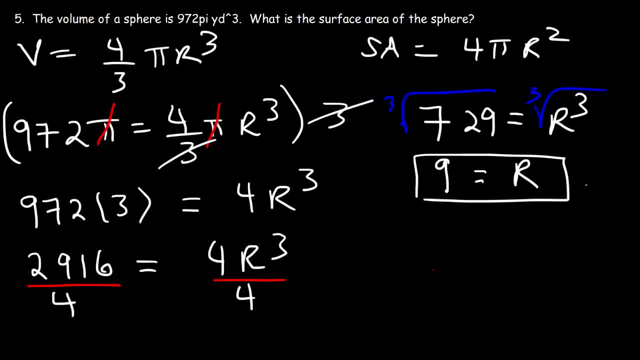 is equal to R. so now that we have the value of our, we can plug it in to the second equation. so the surface area is going to be 4 pi times 9 squared. 9 squared is 81, that's 9 times 9, and 4 times 81. if you multiply 4 times 8, that's. 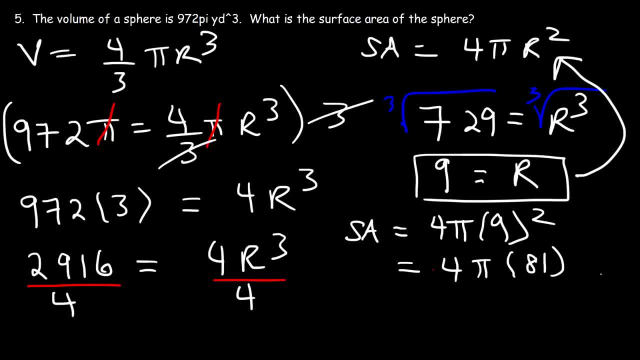 32. so 4 times 80 is 320, and then 4 times 1 is 4. when you add 4 and 320, that will give you 324. so the surface area is 324 pi square yards, and so that's the final. 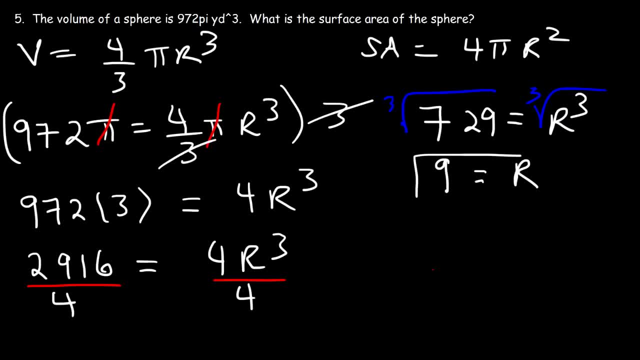 That's equal to 9.. So 9 is equal to r. So now that we have the value of r, we can plug it into the second equation. So the surface area is going to be 4 pi times 9 squared. 9 squared is 81, that's 9 times 9.. 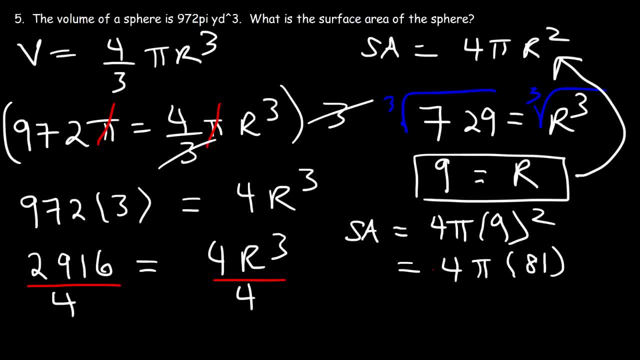 And 4 times 81,. if you multiply 4 times 8, that's 32.. So 4 times 80 is 320.. And then 4 times 1 is 4.. When you add 4 and 320, that'll give you 32.. 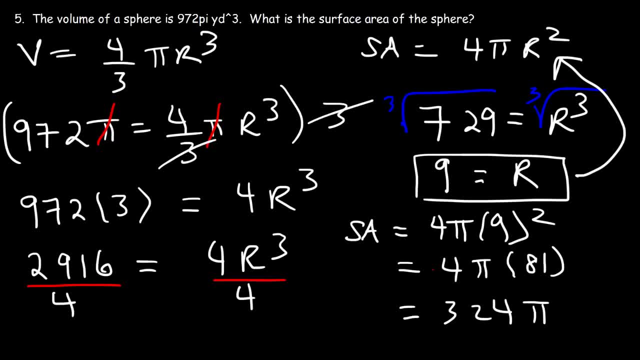 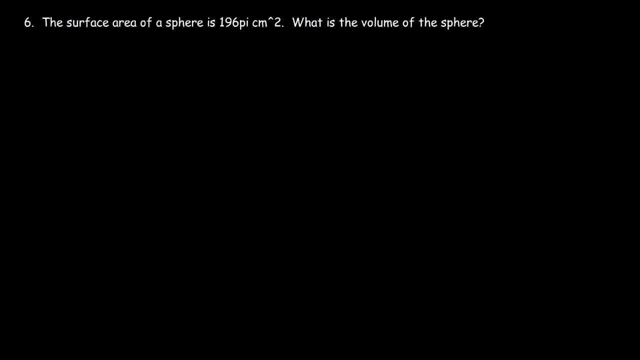 So the surface area is 324 pi square yards, And so that's the final answer for this problem. Here's another problem that's similar to the last one, but not exactly the same, So go ahead and try it for practice. So we're given a surface area this time instead of the volume. 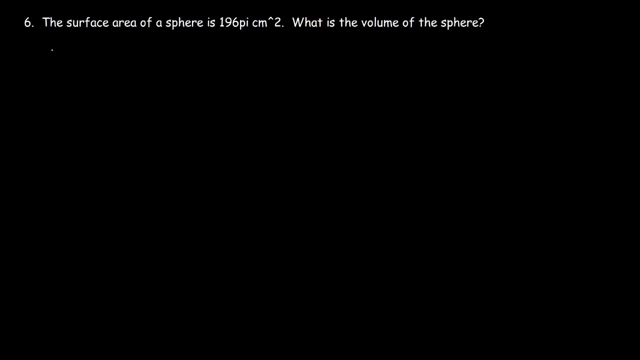 And we want to find a volume instead of the surface area. So let's start with this equation. We need to calculate r first, just like we did before. The surface area is 196 pi, So let's cancel pi and let's divide both sides by 4.. 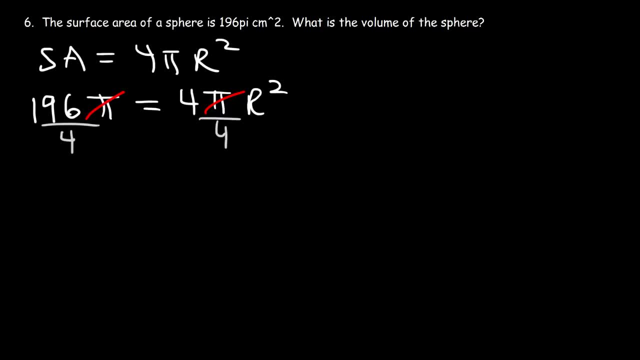 196 divided by 4 is 49.. So 49 is equal to r squared, And if we take the square root of both sides, r is equal to 7.. So now that we have that, we can use this equation to find the volume. 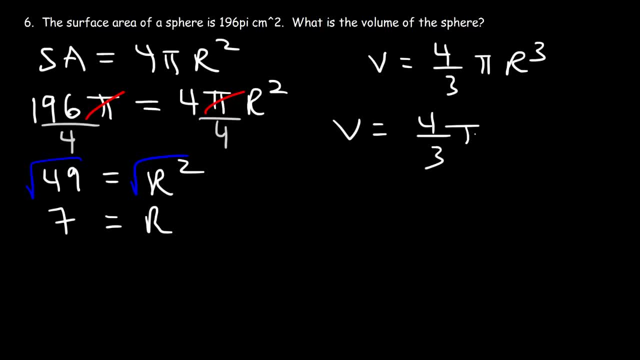 So all we need to do is replace r with 7.. 7 to the third power, that's 7 times 7 times 7.. So that's basically 49 times 7.. That's 343.. 343 is not divisible by 3.. 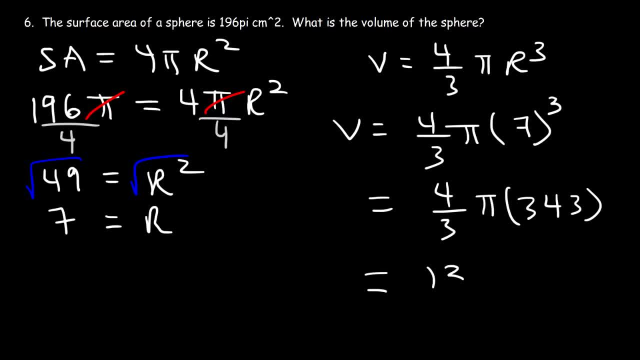 We can multiply it by 4.. So the final answer is 1372 pi divided by 3 as a fraction, And let's not forget the units. The units are cubic centimeters, So that's how you can basically find the volume if you're given a surface area.